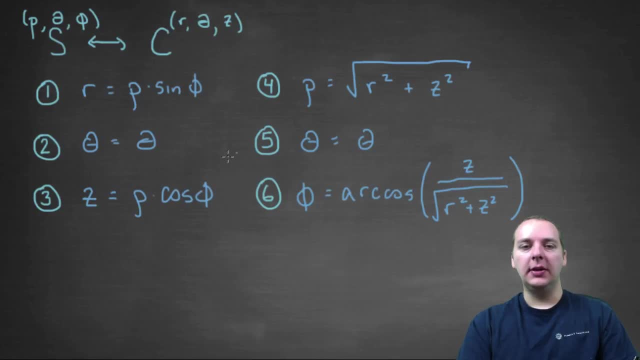 where they come from, because it's kind of interesting to see where all these different equations come from. So I'm going to hide these right here and we're actually going to see where these come from next. If you want to stay with us, we'll love it. if you. 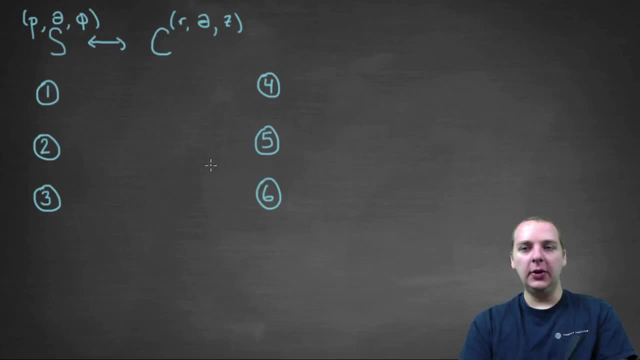 stayed with us. If not, you can go on to the example videos. Alright, so let's see here. On the first set of three, we're going to assume that we're going to have a three dimensional equation, that we're given rho, theta and phi and we're going to try to find r? theta. 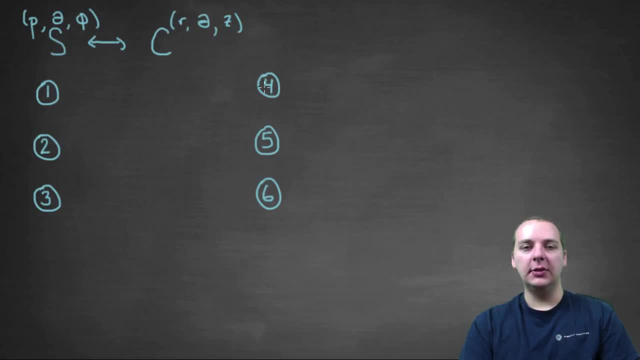 and z, And then the second set of three equations: four, five and six. we'll do the reverse. We'll say that we're provided r, theta and z and we've got to find rho, theta and phi. 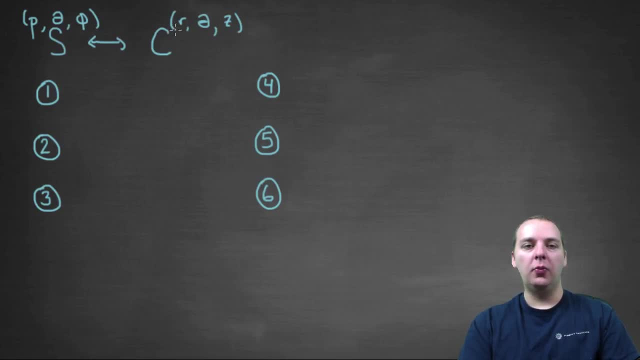 Alright. so how do we do this? first, If we're given an r, a theta and a z, how do you find, let's say, rho? If you bear with us, this is the most complicated of the six. So if you stick it out through the first equation, the other five will take no time at all. But 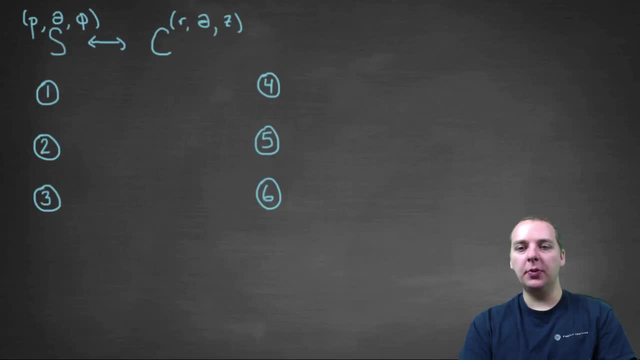 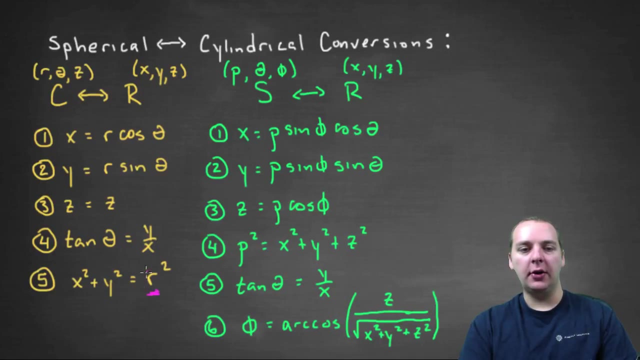 the first one is a little hairy, Alright, so here's what we're going to do. We're going to look at our old equations and I see a r, an r. here's an r. r squared equals x squared plus y squared. And then, in the green list, I see an equation for x and an equation for. 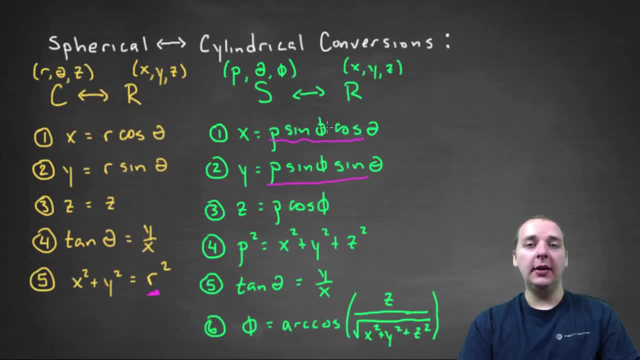 y. And then in the green list I see an equation for x and an equation for y, And then in the green list I see an equation for y that are in terms of rho, theta and phi, And so it sounds perfect. So we're going to take x squared plus y squared and set it equal. 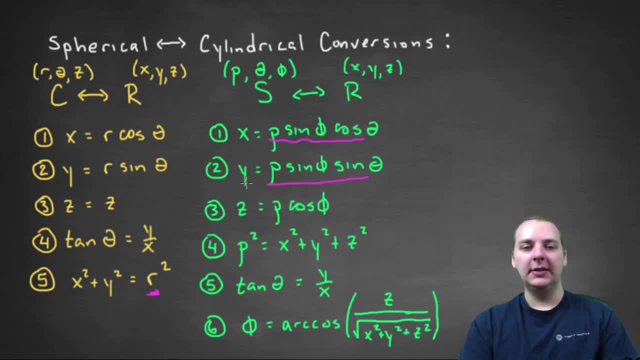 to r squared, But I'm going to use these instead of x and y. So if I can squeeze this in somewhere, I will try to do that. So we'll have rho sine phi cosine theta squared, that's x squared Plus rho sine phi sine theta squared. X squared plus y squared equals r squared. 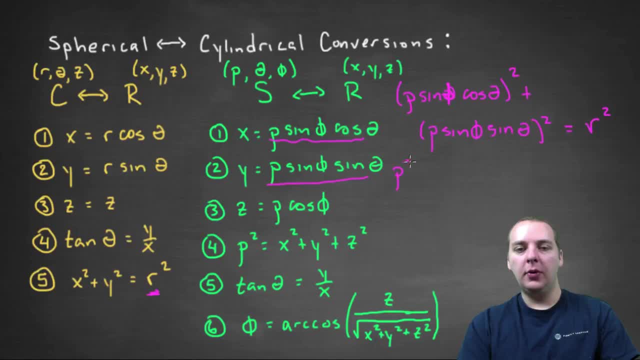 Alright, let's square everything. We'll have: rho squared times sine squared phi times cosine squared theta Rho squared sine squared phi sine squared theta equals r squared. Look at these two terms on the left hand side of the equal sign. They both have a common factor of rho squared. 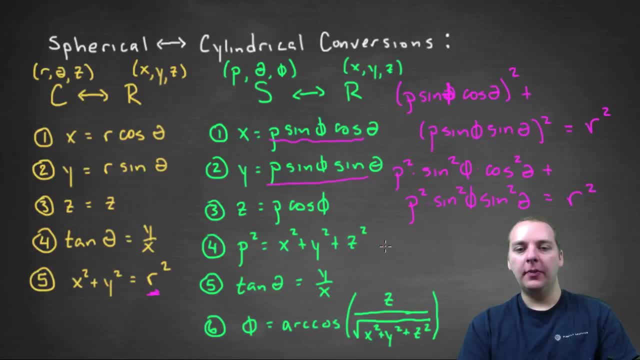 sine squared phi. Let's factor that out. Rho squared times, sine squared phi times what We'll have? cosine squared theta plus sine squared theta. But wait a minute, Cosine squared plus sine squared, that's one, isn't it? That's a trig identity. So actually we'll just have 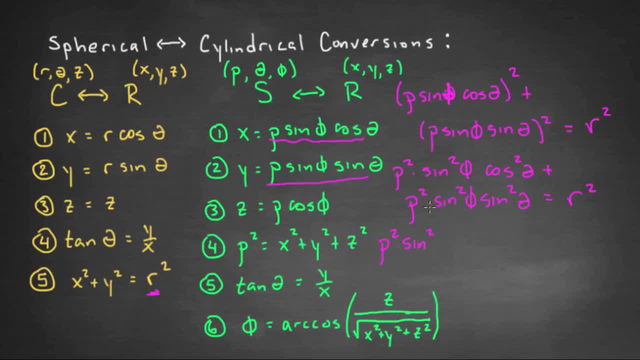 rho squared times, sine squared. Actually, I made a typo, my mistake. It should be sine squared phi, not sine squared theta. I hope I said it right, but I wrote it incorrectly. But cosine squared theta plus sine squared theta would be one, And so that would be equal. 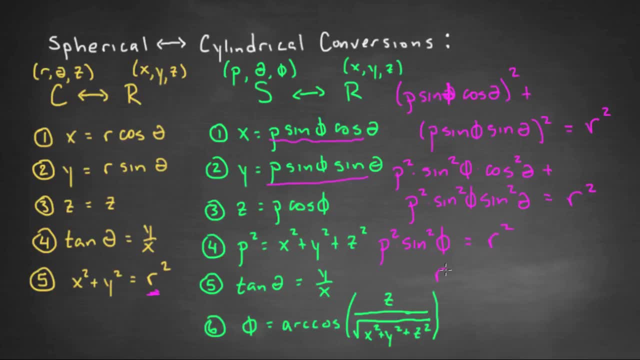 to r squared, And so you would have r equal to rho sine phi And r. let's assume r is positive and rho is positive, So we would have r equals rho sine phi, And since phi is zero to 180, and the first and second quadrant signs already positive, so we can just take the square root. 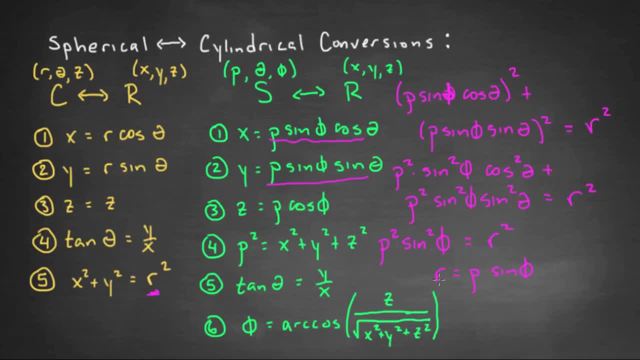 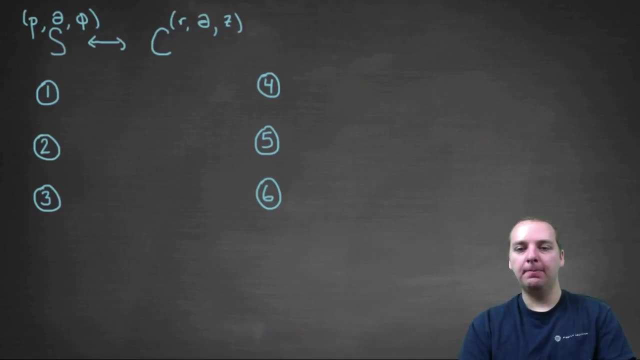 of both sides here. So there you go. That's your conversion we're after. If you want an r value, but all you have is rho squared. If you want to multiply both theta and phi, then we've got it. So here we go. So we would. 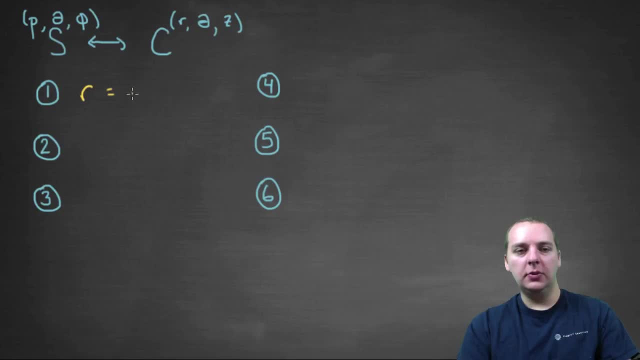 have. let's see here: R equals rho times sine of phi. So given a rho and a phi, we can find r. Alright, that was a long one. If you made it through that one, congratulations. The other five are very fast and very easy. Um, if we were given. 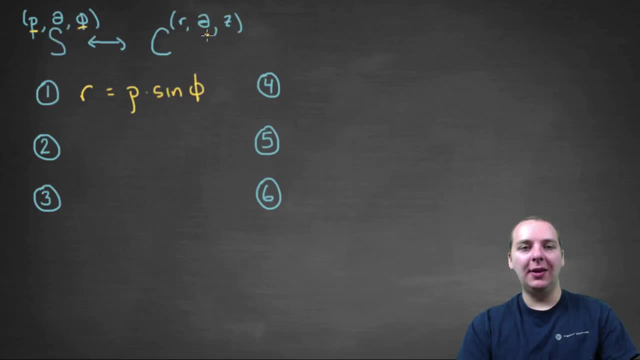 given a row theta and phi, and we wanted theta. easy done. the theta's are the same, So you'll take your theta and that will be your new theta. So if your theta in spherical coordinates was pi over four, the theta in cylindrical 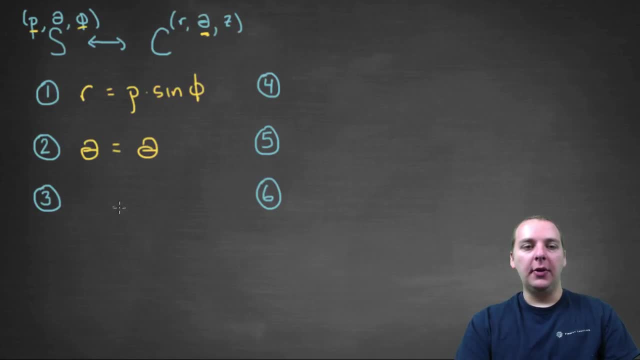 form would be pi over four. For the third equation: if you want, we have r, we have theta. if you want z, that's done, that's immediate. Now we can cheat a little bit. If we're given row theta and phi, we can find z. 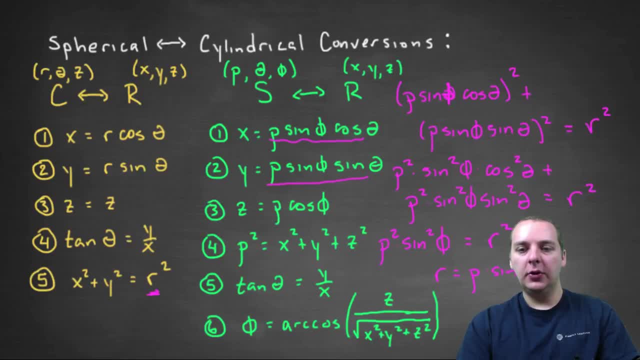 Let's look back at our old equations here. Look at this one in orange that I'm boxing in right here. right here, Given a row and a phi, we can find our z value. Rectangular form has a z and cylindrical form has a z. so it's the same formula. 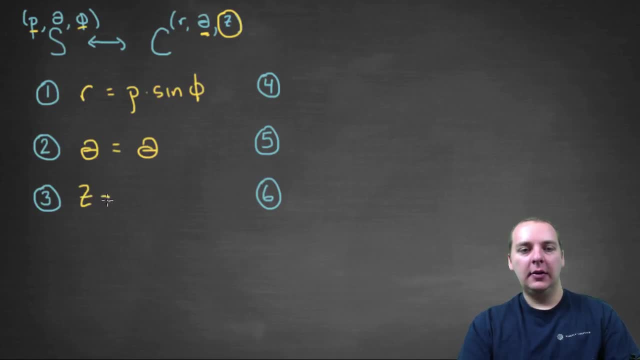 So we'd have z Equals row cosine phi. So we've converted r, theta and z. Now let's go the other direction and these three will be also pretty fast. Let's assume now we're given row. I'm sorry, r, theta and z and we want row. 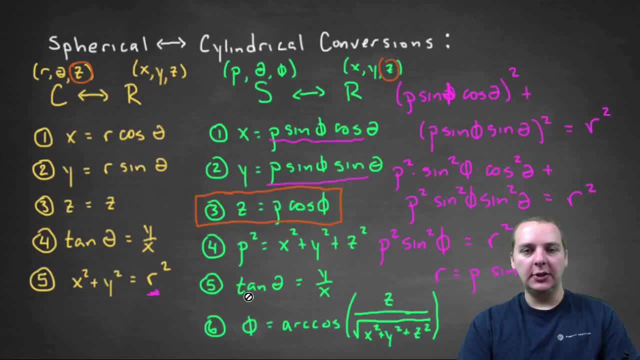 So let's look back at our old equations and see if there's anything we can kind of cheat with a little bit. Um, Let's see, Let's see, Let's see. Alright, Look at um, Look at this one right here in: uh, red. 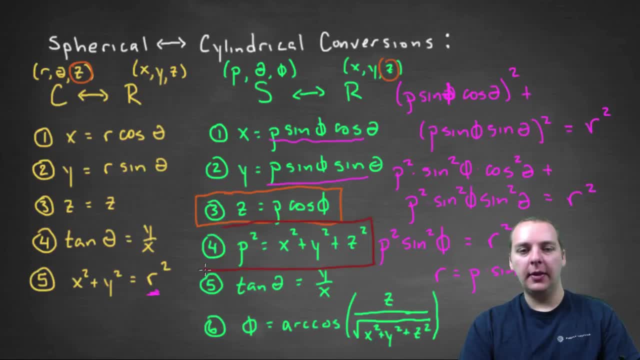 Look at this one. I'm boxing in in red right here. Row squared equals x squared plus y squared plus z squared. Now you say: well, Devin, you can't use that. That's an x and a y, That's not cylindrical form. 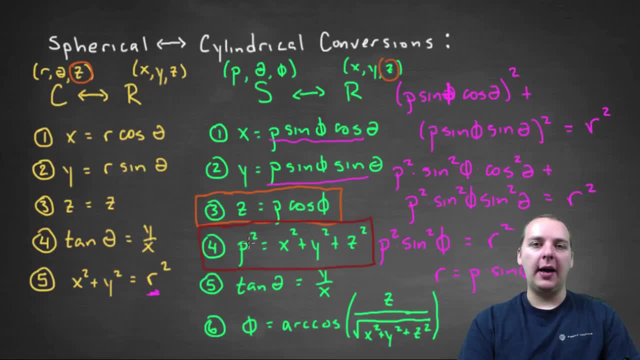 That's rectangular form. Well, row is okay to have because that's spherical. Z Z is okay to have because that's cylindrical. But think about the x squared plus y squared. Can you convert that to cylindrical? What is x squared plus y squared? 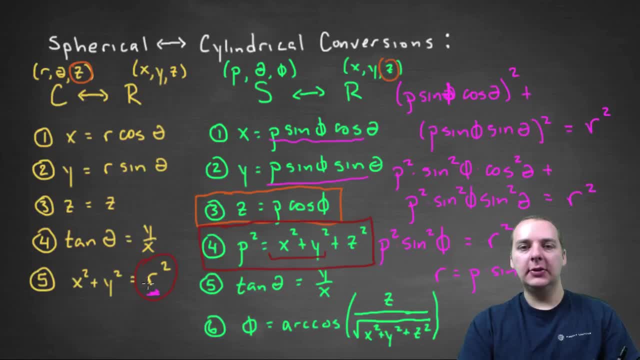 Hint, hint, It is r squared, So let's, let's do this and I'll. I'll do this in white up here in the corner. You can write this as: row squared equals not x squared plus y squared plus z squared, but 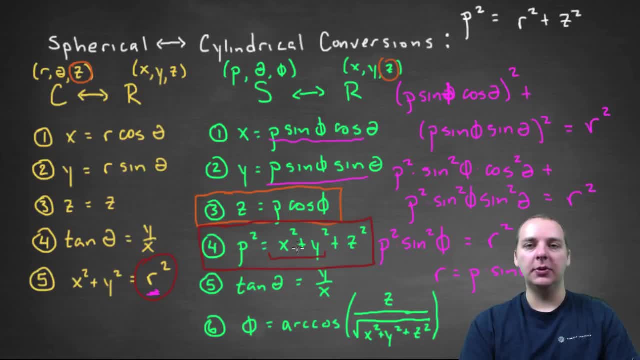 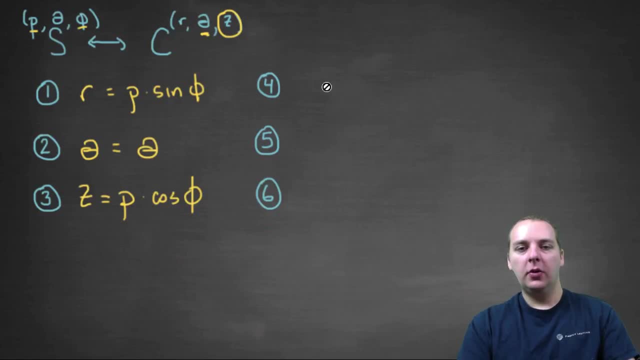 r squared plus z squared, Cause I I just took out the x squared plus y squared, Switched it for r squared. Okay, so row would be the square root of not x squared plus y squared plus z squared, but r squared plus z squared. 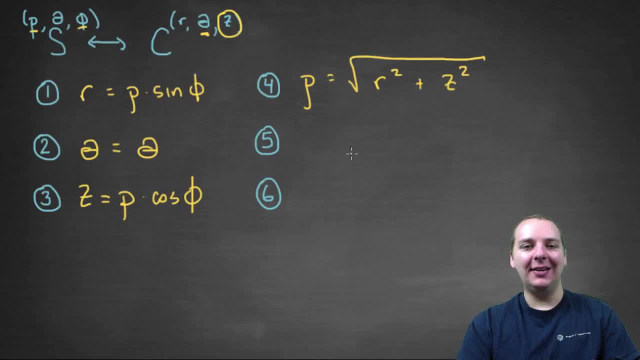 Number five, just like number two, if you're given a theta in cylindrical, that's the same as theta in spherical. So theta equals theta. Alright, now our last one, last one. We've got a row. we've got a theta. 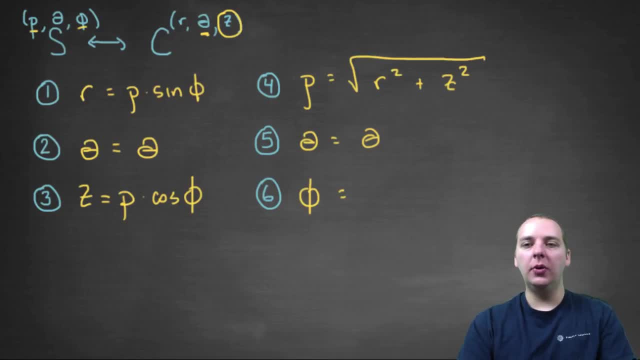 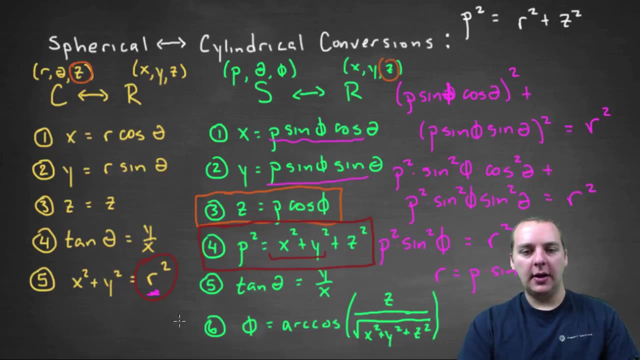 How do you get phi? How do you get phi? Let's look back at our old equations. Was there any old equation that had a phi? I think there is. How about this guy right here in blue with the star right here? Phi is this. 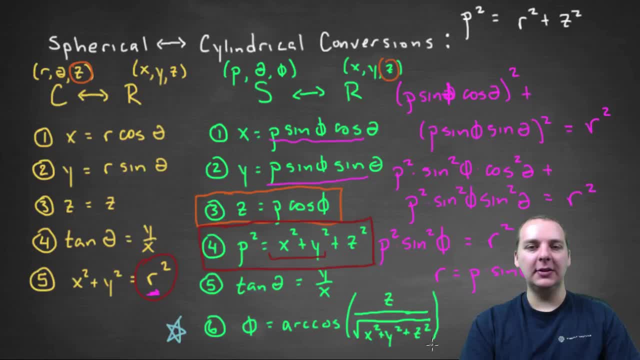 But then you say: well, wait a minute, Devin, I'm okay with the z. The z is fine, Z is cylindrical. X squared plus y squared, that's not cylindrical. Oh, but wait, we have that same trick as before, right here. 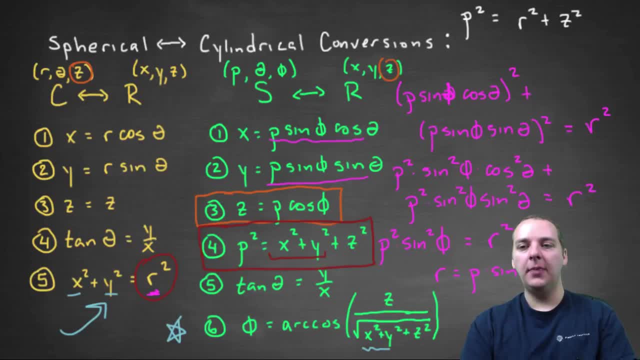 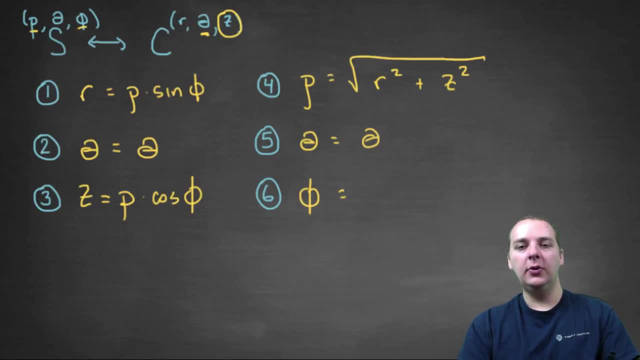 X squared plus y squared is r squared, So we can just swap that out and we're done. So if it feels kind of like cheating, it kind of is We're just using old stuff to find new stuff. So we'll have arc cosine of z over the square root. 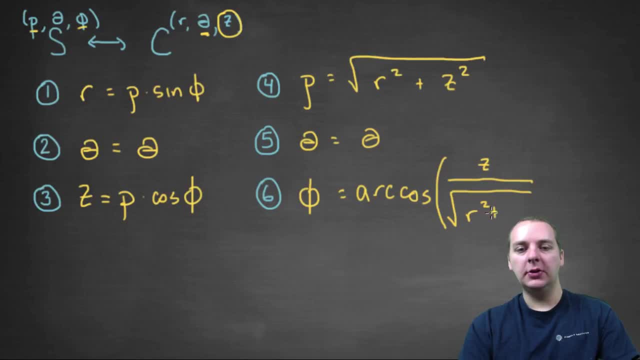 Not x squared plus y squared, Not y squared plus z squared, But just r squared plus z squared. So we can go both directions now: from spherical to cylindrical and cylindrical back to spherical. So that completes the circle. We have three different forms.